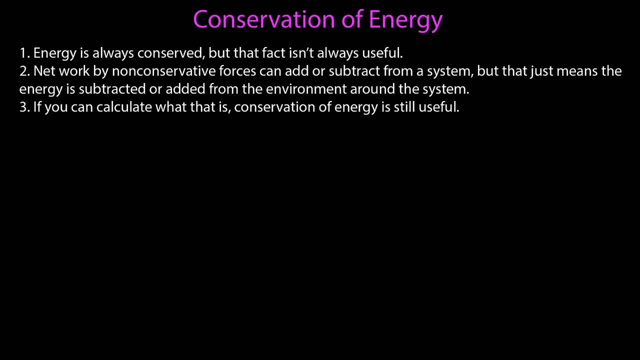 That energy still exists somewhere. Net work by non-conservative forces can add or subtract from a system, but that just means the energy is subtracted or added from the environment around the system. For example, take something sliding under friction. So the friction is a non-conservative force which is removing energy from the system, removing the kinetic energy. 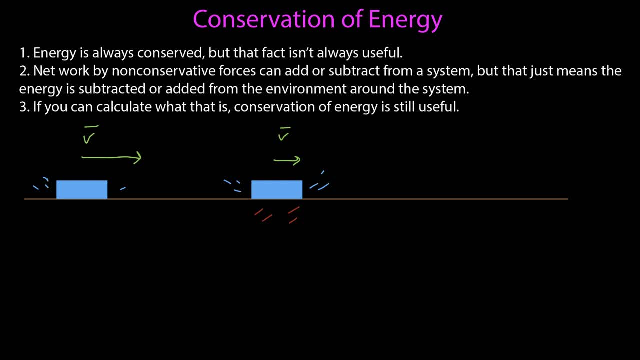 But that energy is going into the thermal energy of the ground. The ground is heating up due to that friction. In the end the object is at rest. it has lost all of its kinetic energy, But that energy is now contained into the thermal motion of the particles of the environment. 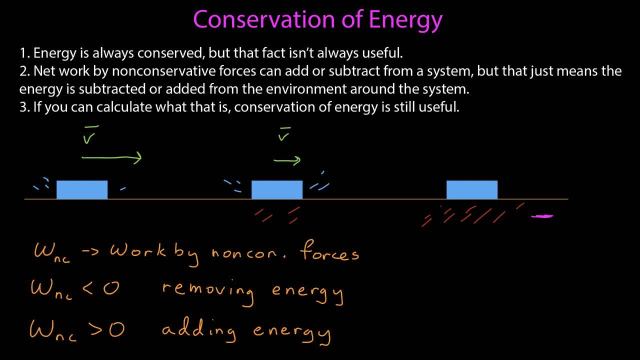 So let's talk about the work done by non-conservative forces, Because if you can calculate what that is, then conservation of energy is still useful to solve problems. So I've labeled work done by non-conservative forces As this: W with a subscript, NC. 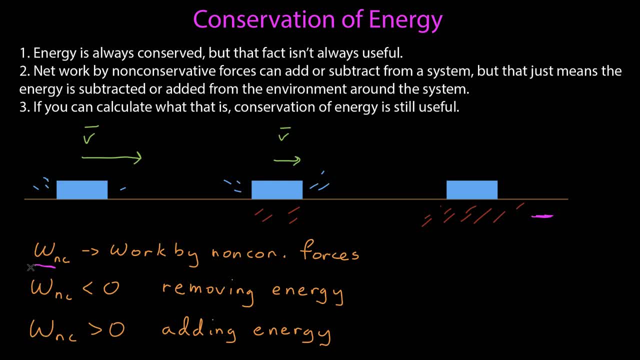 First of all, remember that if it's removing energy from the system, then the work done by those non-conservative forces is less than zero. If it's adding energy to the system, then it's positive. So the question is how to account for that when we apply conservation of energy. 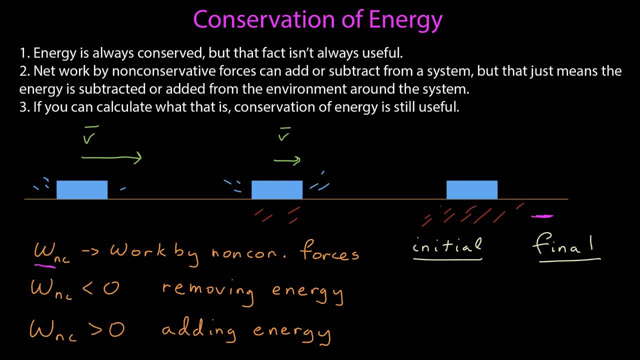 Previously I said: look at two points in time And you add all of your initial energies and all of your non-conservative forces. And you add all of your initial energies and all of your final energies, And they should be equal. And when we had conservation of mechanical energy, those energies were our initial potential and kinetic energies and then our final potential and kinetic energies. 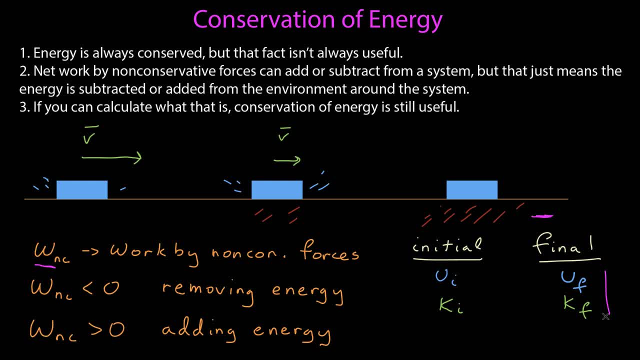 So where to include this work done by non-conservative forces? This energy isn't really initial or final. It's during The work being done by non-conservative forces occurs between the initial and final time, And you can include it, in fact, either place. 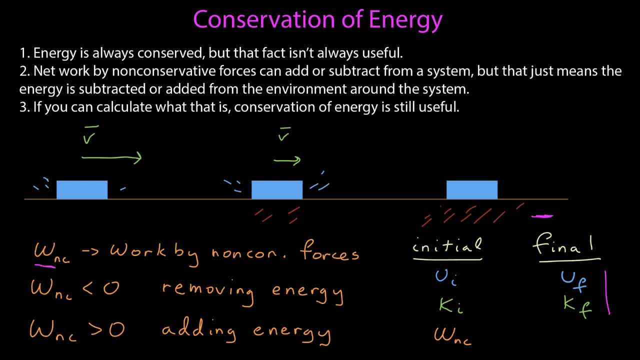 For example, you could just list it with your initial energies. This is the initial energy that you start with, And if it's less than zero, then it would subtract from that initial energy And the result would be equal to your final energy.